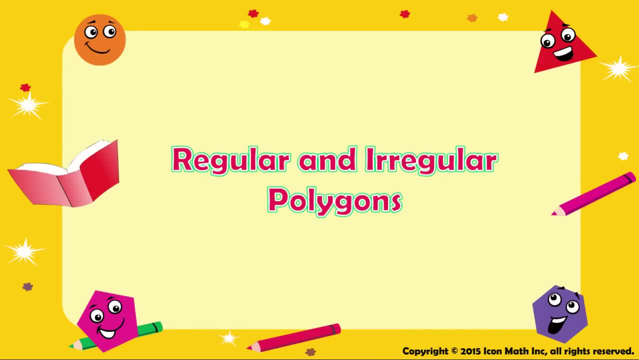 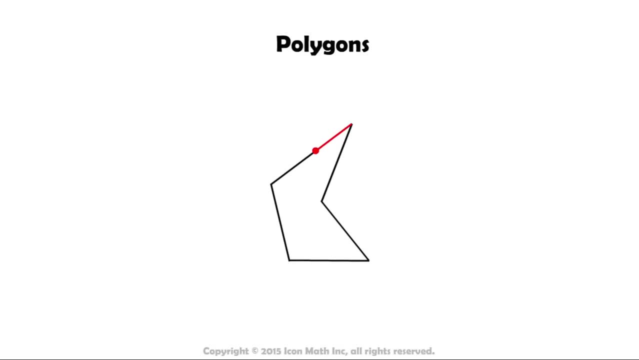 Regular and Irregular Polygons. As we learned before, a polygon is a closed two-dimensional shape made up of line segments. only If we have these two polygons, what can we say about their properties? Let's talk about the first one. The sides length of this square are equal, as well as the size of its four angles, because they are all right angles. 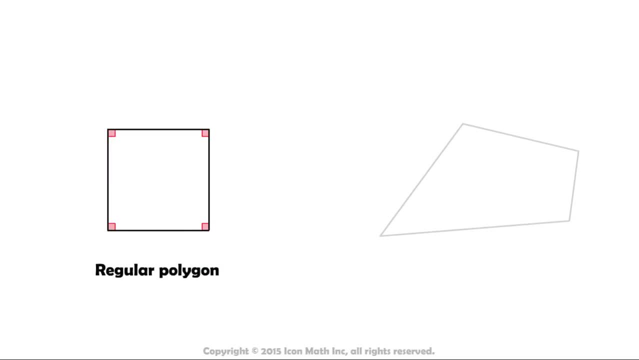 This kind of polygon is called a regular polygon. So a regular polygon is a polygon with equal sides and equal angles. Now let's look at a regular polygon. Let's have a look at the second polygon. It is obvious that the sides of this polygon aren't equal, and neither are the sizes of the angles. 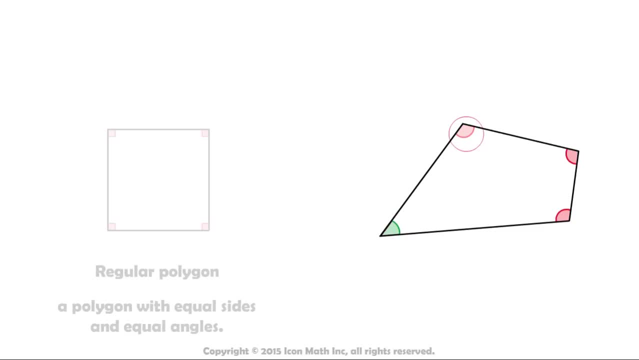 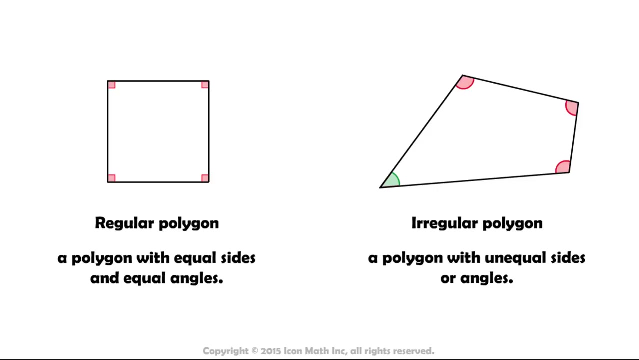 For instance, we have an acute angle, but the rest of the angles are obtuse. Therefore, this polygon is not regular. We call such polygons that don't have equal sides or angles irregular polygons Thery прямо, and the only way to call them regular is to ask a question. 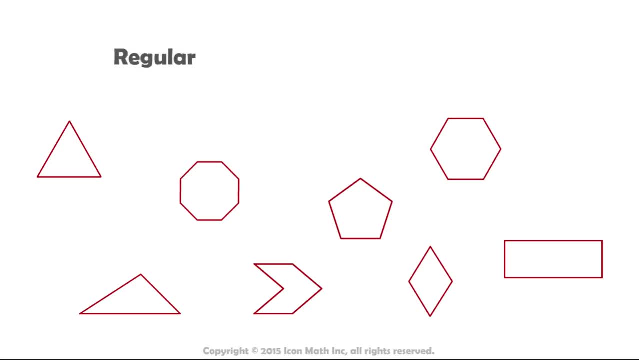 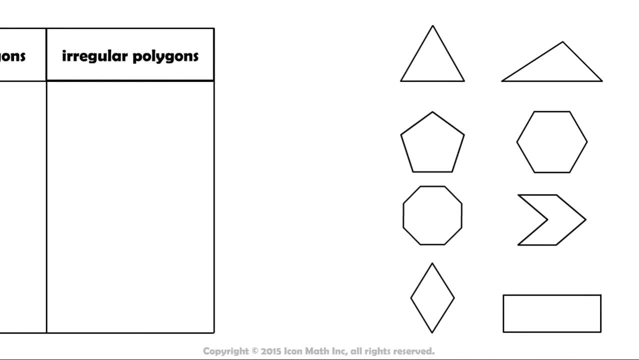 Among these polygons, can you tell which ones are regular and which are not? Let's check together and sort these polygons in the following table. Look at this triangle. It has three equal sides and three equal angles, so it is a regular polygon. 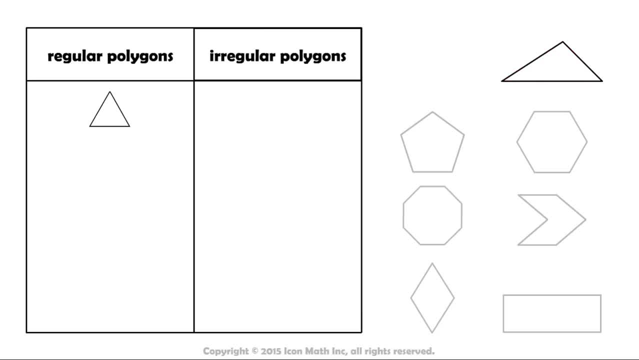 But this second triangle is not regular because neither its sides nor its angles are equal. What about this pentagon? The sides of this pentagon are equal. Notice that the opening between each two intersecting line segments within the shape is the same, which means: 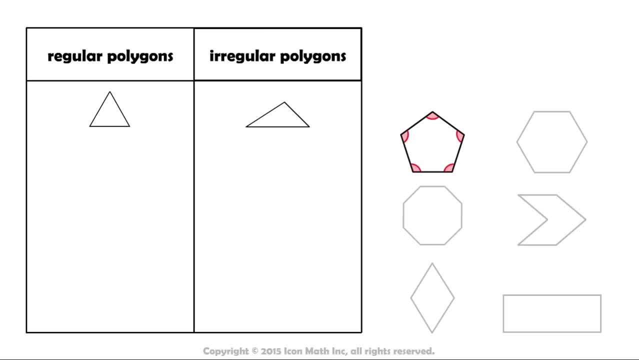 that all those angles are equal. So this pentagon is regular. Similarly, this hexagon and this octagon are both regular polygons. Now what about this one? As you can see, all its sides are equal, But still it is not regular. 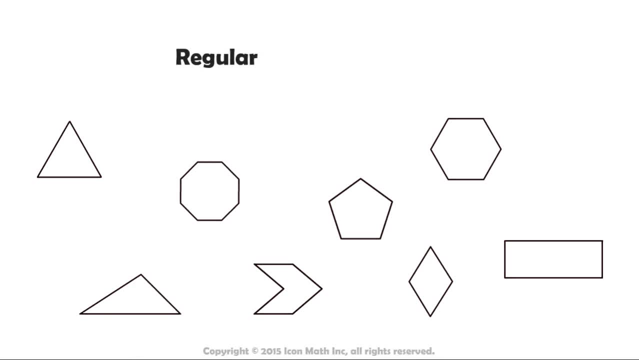 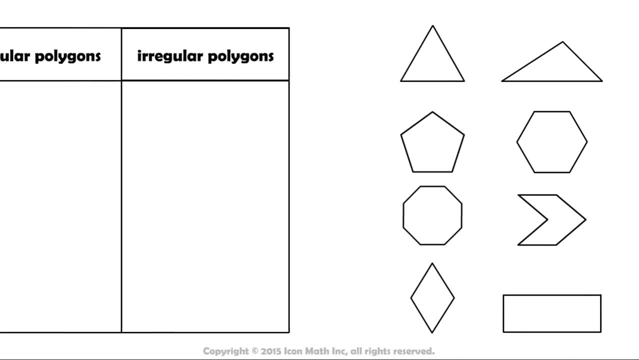 Among these polygons, can you tell which ones are regular and which are not? Let's check together and sort these polygons in the following table. Look at this triangle. It has three equal sides and three equal angles, So it should be equal, but also more than equal. It is according to this table's quadratic rules and it has three equal angles and three equal sides. So we can say that the first one has three equal sides and the second one has three equal angles. So if we compare these three polygons, then we have the same thing. 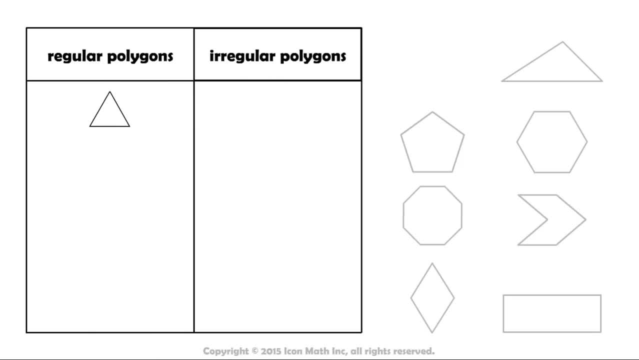 Now let's do a little exercise. So it is a regular polygon, But this second triangle is not regular because neither its sides nor its angles are equal. What about this pentagon? The sides of this pentagon are equal. Notice that the opening between each two intersecting line segments within the shape is the same. 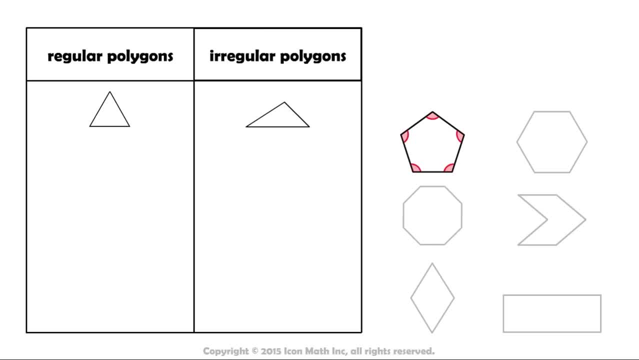 which means that all those angles are equal. So this pentagon is regular. Similarly, this hexagon and this octagon are both regular polygons. Now what about this one? As you can see, all its sides are equal, but still it is not regular, because the angles 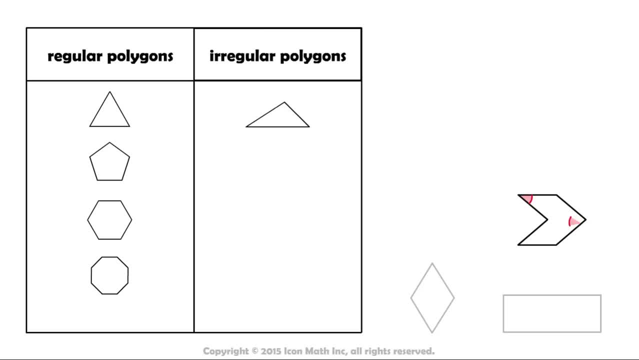 within this polygon are equal. This rhombus has equal sides, but its angles are not equal, so this shape is also an irregular polygon. This rectangle is irregular. Although the four angles are equal, they are not equal. In this lesson, you learned how to identify the characteristics of regular polygons. 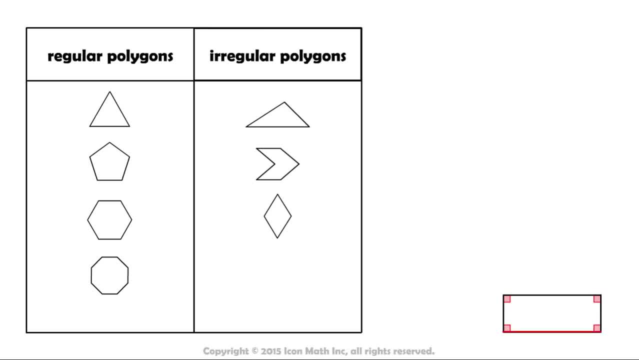 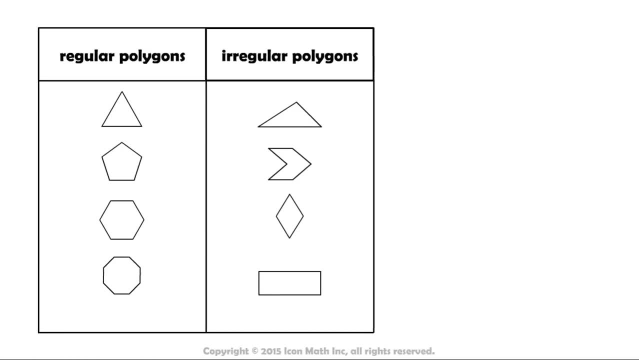 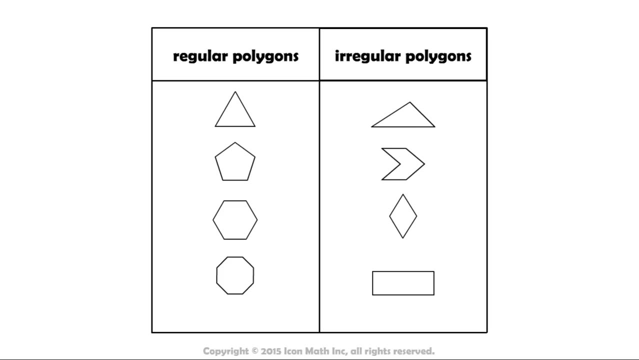 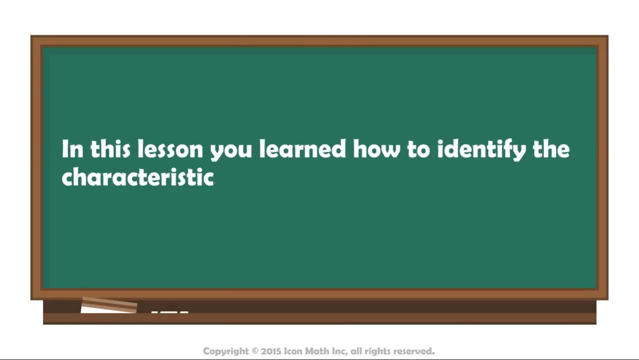 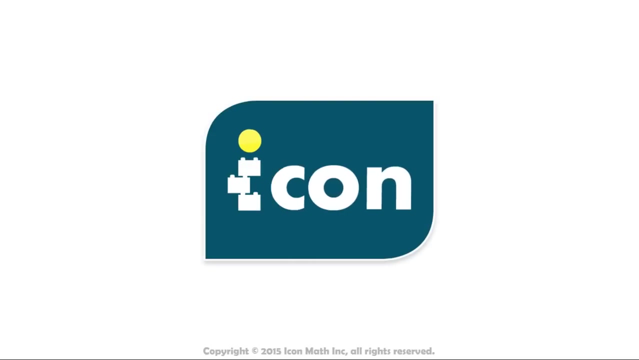 In this lesson you learned how to identify the characteristics of regular polygons. You will probably realize that the được a vectors with numbers. If you likes this video, dele carva, you can like, comment, share. Kil gray, I'll see you next time. Have a nice day, Bye.